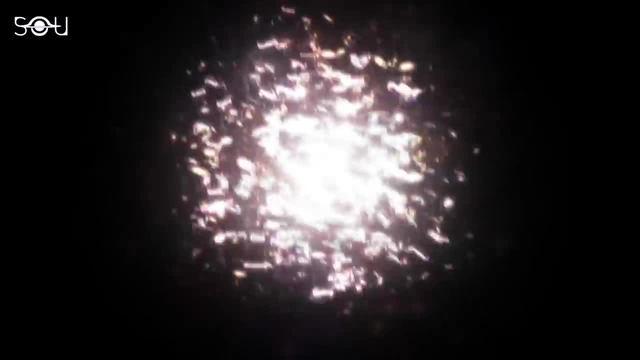 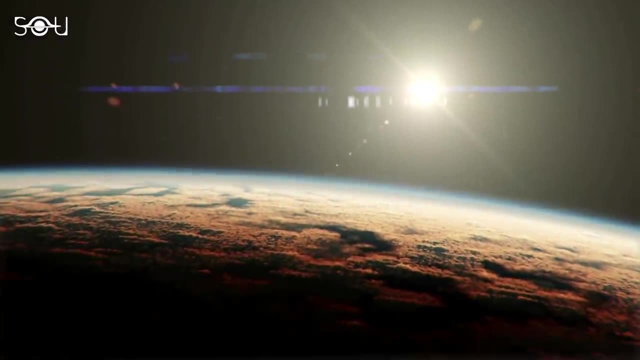 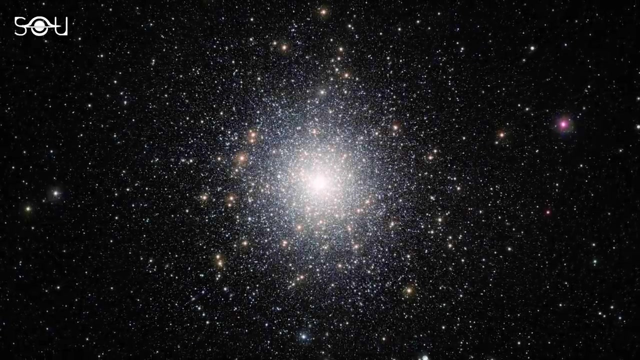 about 4 billion years old, But Earendel was there in the first 900 million years of the Big Bang. This means that this star is about 8.2 billion years older than the Sun and the Earth. So far, the smallest objects observed at these distances were star clusters embedded. 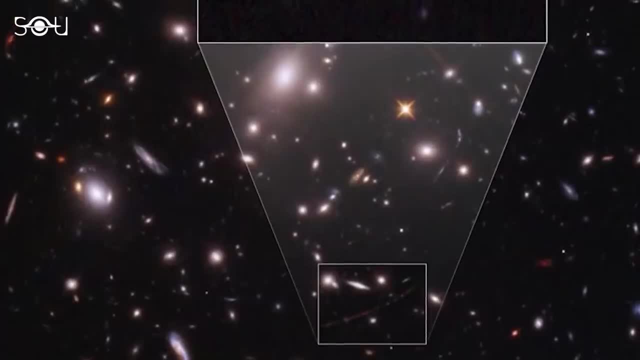 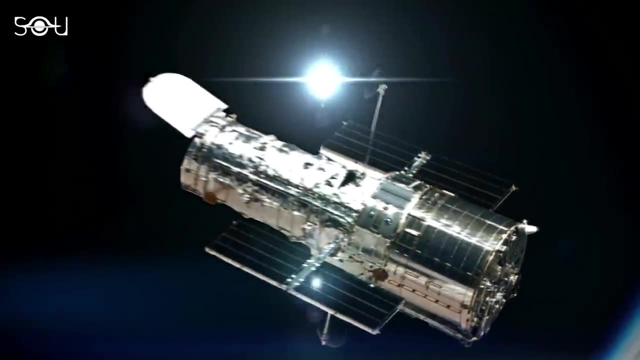 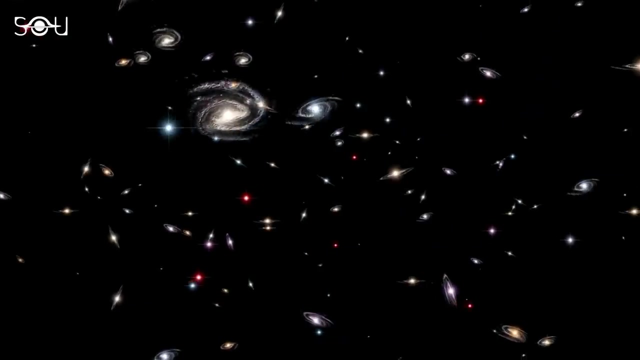 in distant galaxies, But Earendel is the first isolated star found at such a large distance. This star was discovered by chance using the Hubble Space Telescope. Hubble first observed the star's parent galaxy that was gravitationally lensed by a galaxy. 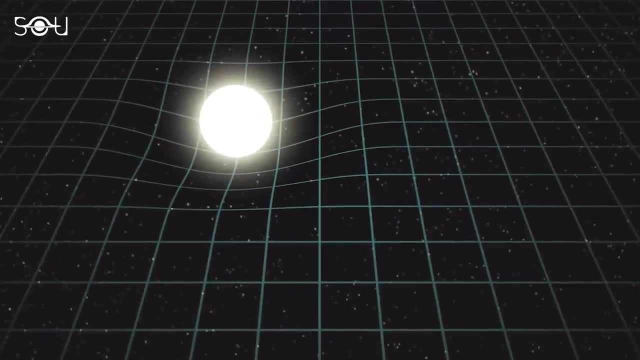 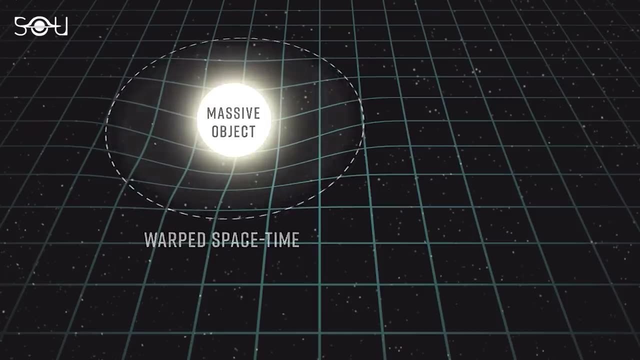 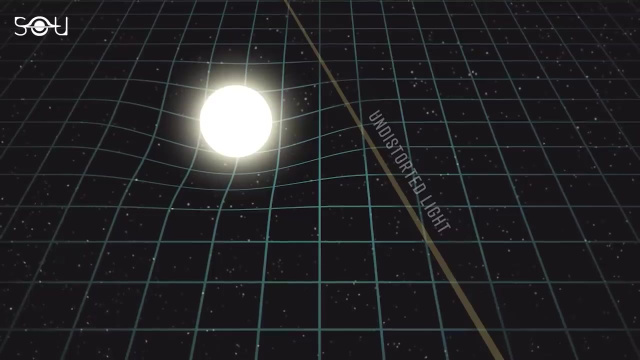 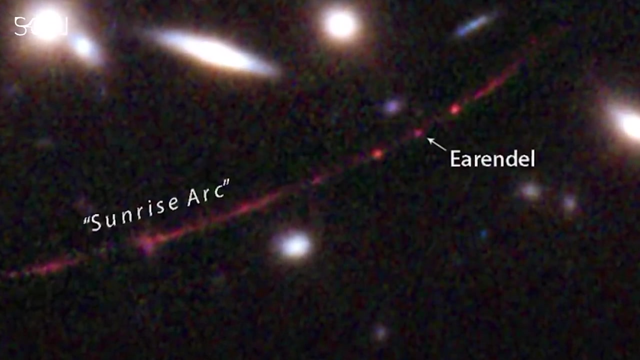 cluster in the foreground. Massive astronomical objects such as galaxy clusters distort the space time fabric around them. As a result of this distortion, the light from the foreground's celestial bodies bends when it passes close to these massive objects. Because of this gravitational lensing, the background galaxy containing Earendel appeared. 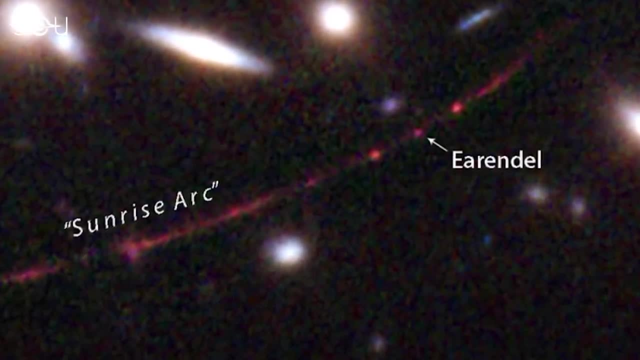 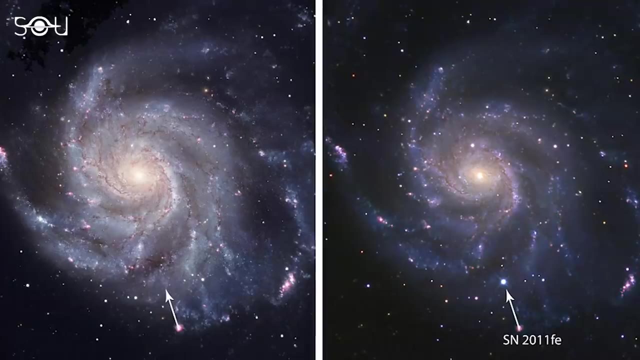 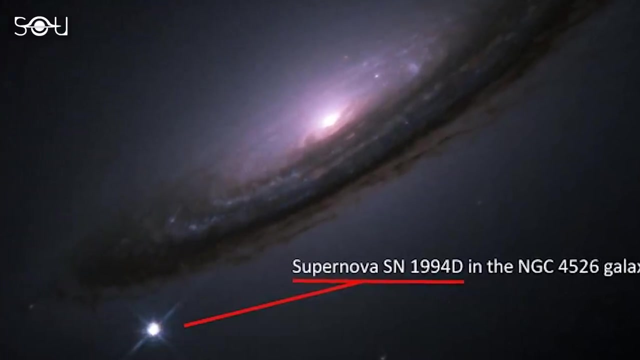 like an arc that the astronomers named the Sunrise Arc, But the team saw a bright object sitting on the edge of the distorted galaxy. Luminous sources in distant galaxies tend to be highly energetic events such as novas supernovas or tidal disruptions caused by black holes. These are 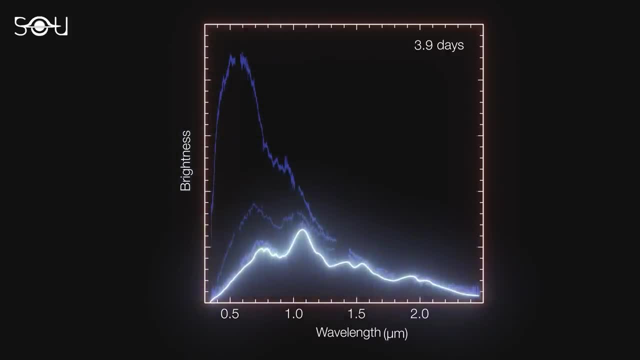 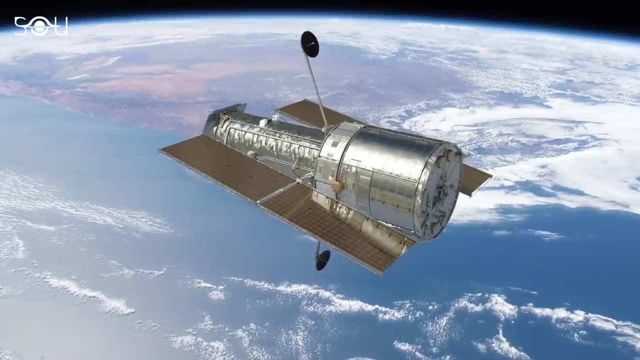 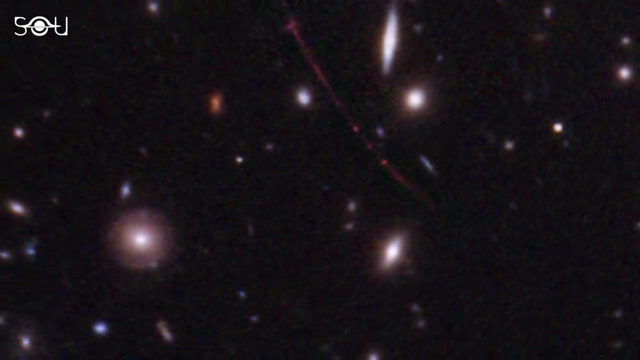 transients that happened to change their brightness with time. However, Hubble's observations showed that the brightness of this object remained constant for over three and a half years. Hence, astronomers concluded that it's a gravitationally lensed bright star in Sunrise. 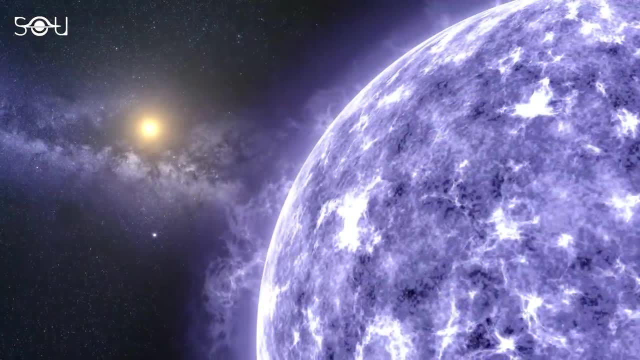 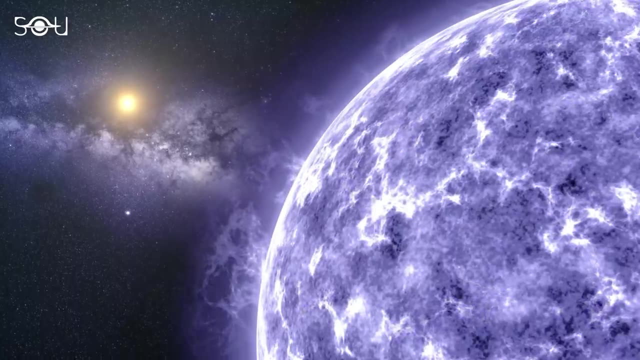 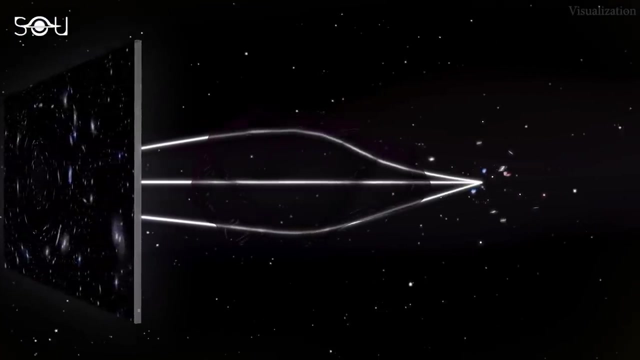 Arc. The research team estimates that Earendel is at least 50 times the mass of our Sun and millions of times as bright, rivaling the most massive stars known. But even such a brilliant, very high-mass star would be impossible to see at such a great distance without the. 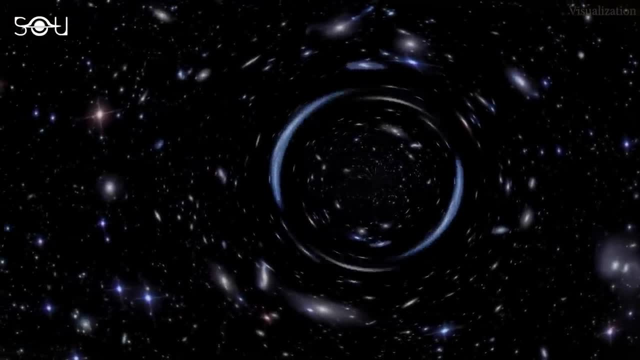 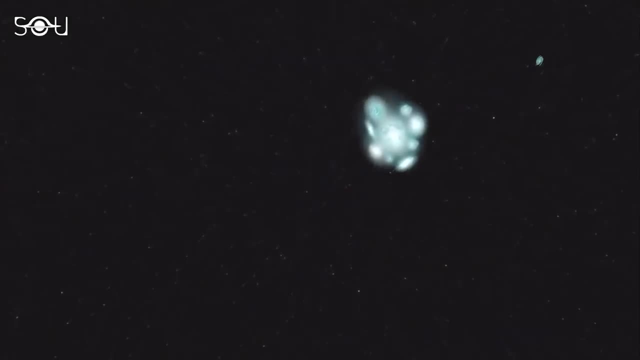 aid of natural magnification by a colossal galaxy cluster sitting between Earendel and us. The mass of the galaxy cluster warps the fabric of space, creating a powerful natural magnifying glass that distorts and dramatically amplifies the light. The mass of the galaxy cluster was so large that it could only be seen by the naked eye. 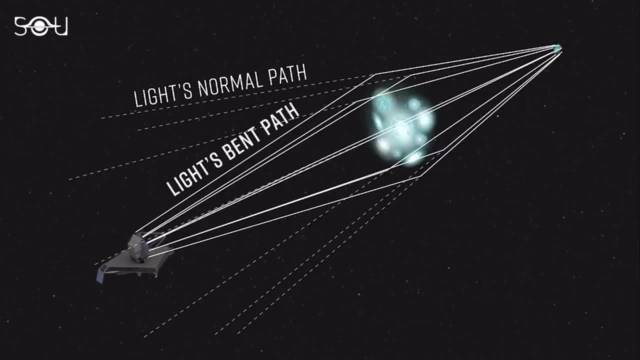 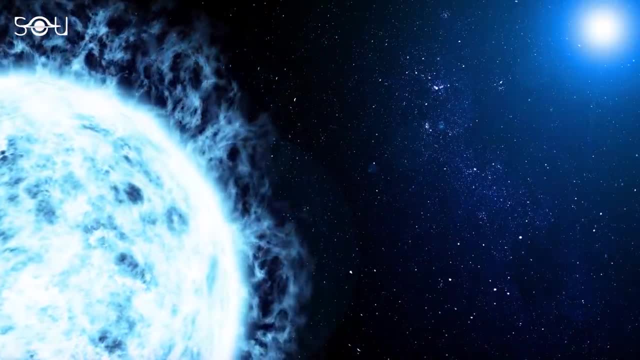 The mass of the galaxy cluster was so large that it could only be seen by the naked eye. The mass of the galaxy cluster was so large that it could only be seen by the naked eye. Given the star's age and the estimates of its mass, it probably no longer exists. Massive. 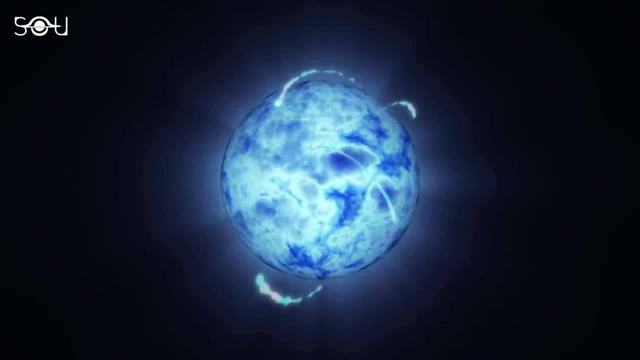 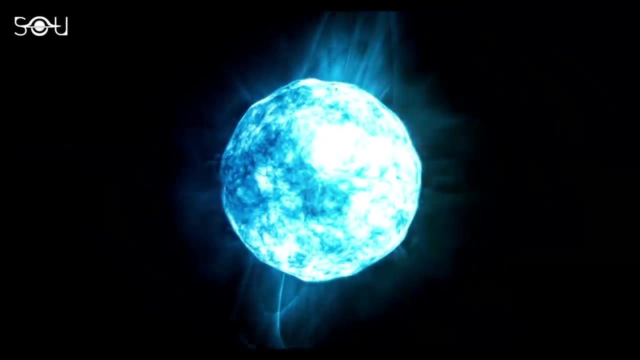 stars such as Earendel use their nuclear fuel much more quickly than small and mid-sized stars. As a result, they have an average lifespan of a few million years, Compared to about ten billion years for sun-like mid-sized stars and up to one trillion years. 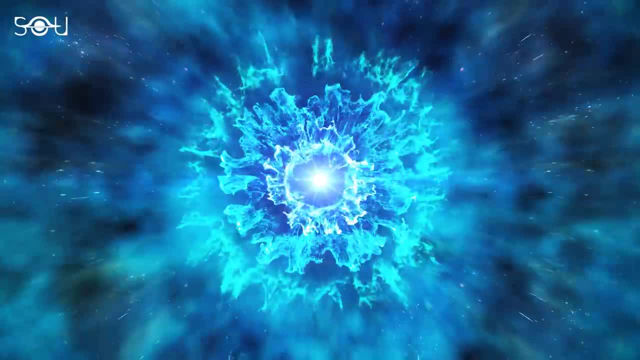 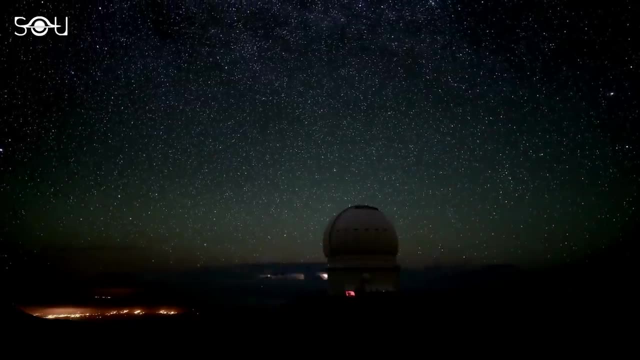 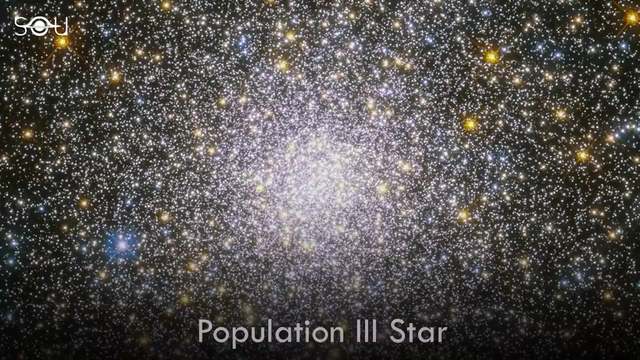 for red dwarfs. Hence Earendel might have died in a fiery explosion billions of years ago. Earendel's discovery is important because it might be the first observation of a population three star that astronomers had been hunting for decades. Primordial nucleosynthesis produced 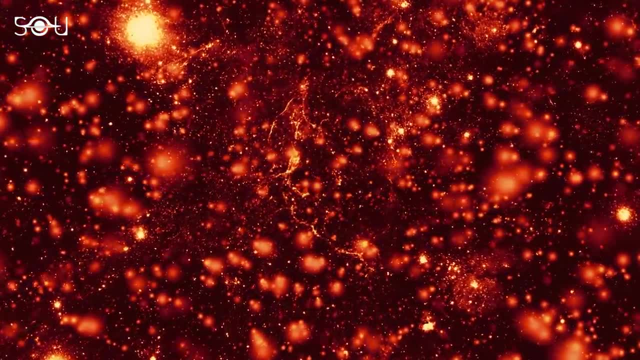 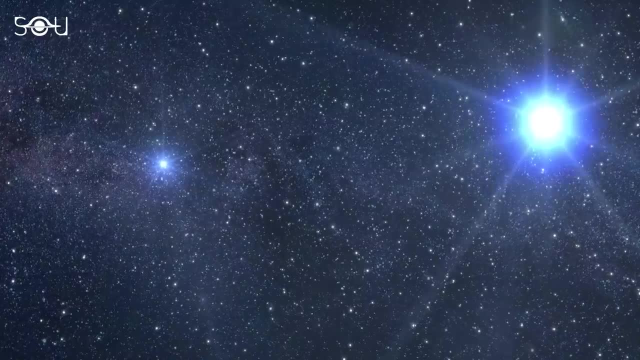 two major chemical elements. Earendel's discovery might be the first observation of a population three star that astronomers hydrogen and helium, The first generation of stars known as Population III stars, had trace amounts of metals and hence a low metallicity In astronomy. any element other 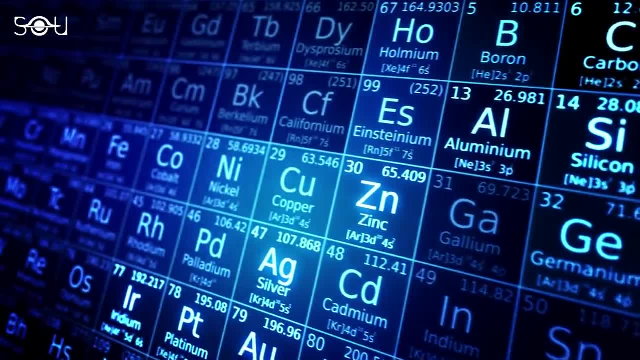 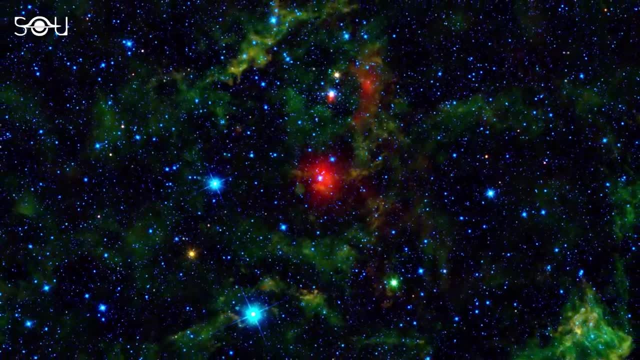 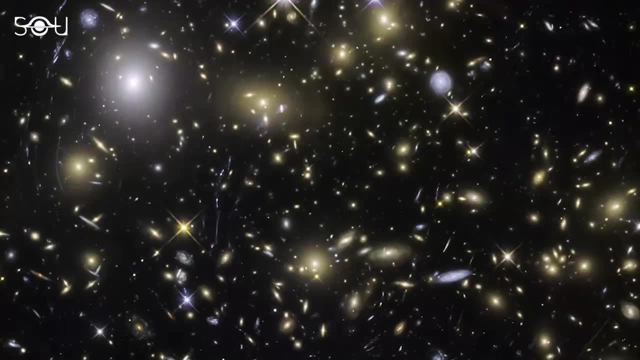 than hydrogen, and helium is referred to as a metal. Astronomers believe that most of the Population III stars have died by now, and the remaining ones are pretty dim and difficult to observe. They're almost impossible to be seen naturally, and most of the candidates have been. 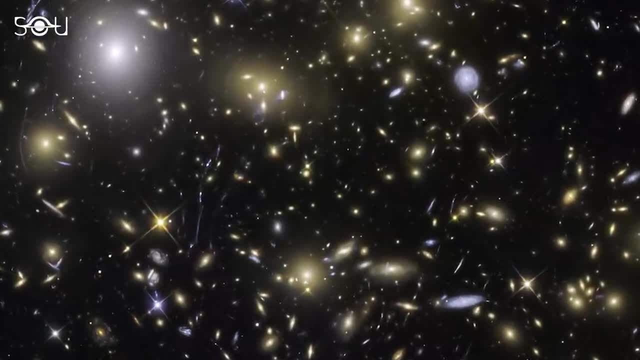 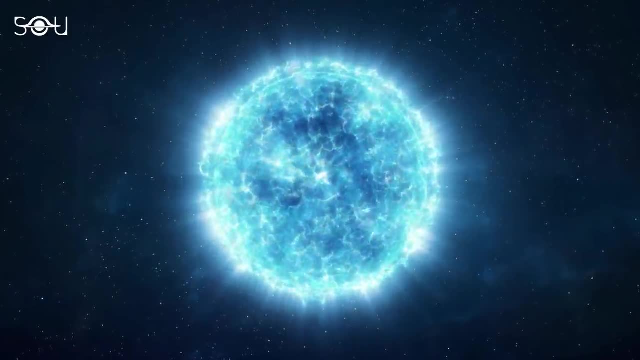 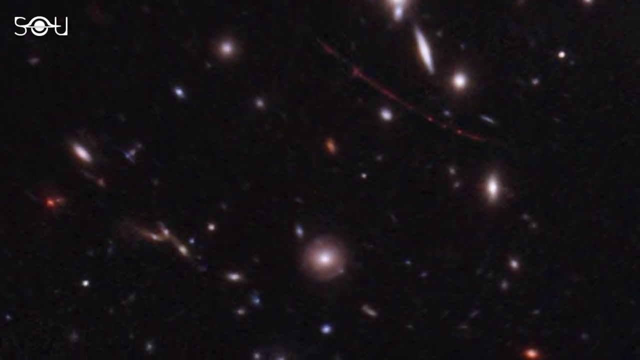 found in gravitationally lensed galaxies, Unlike Icarus, a blue supergiant star. we don't really know about the spectral classification of Earendel. It could even be a binary star system. However, astronomers expect that Earendel will remain highly magnified. 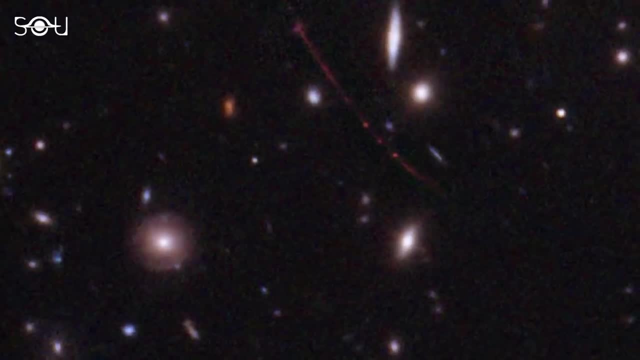 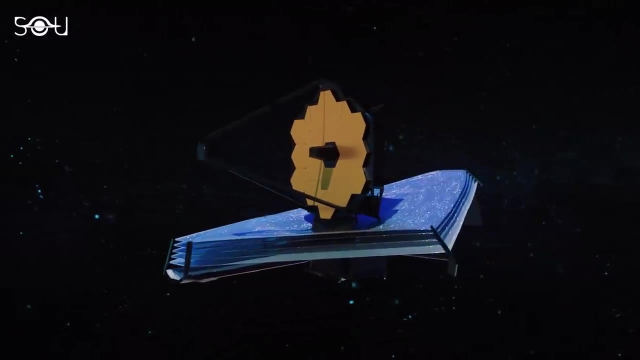 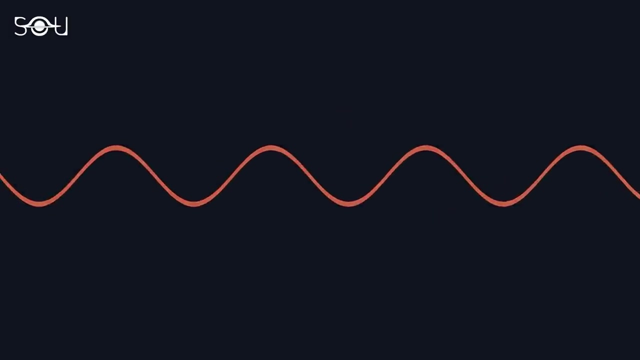 for years to come, and powerful telescopes such as the James Webb Space Telescope will determine its properties. Webb's high sensitivity to infrared light is needed to learn more about this far-flung star, because its light is stretched or redshifted to longer infrared wavelengths due to the universe's expansion. Accurate measurement.